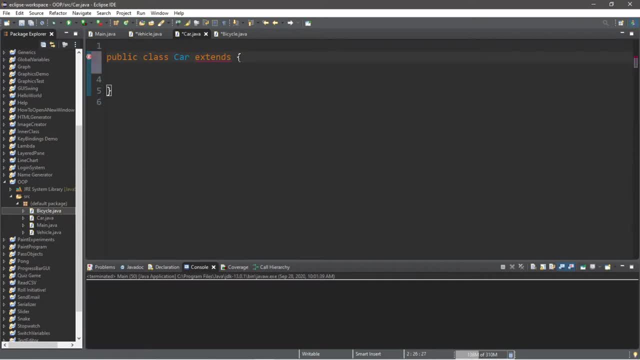 So car extends my vehicle class And we'll do the same thing for bicycle. Bicycle extends vehicle. Now, the car class and the bicycle class are subclasses of the vehicle class, Also known as child classes, and the vehicle class is the super class, also known as the parent class. 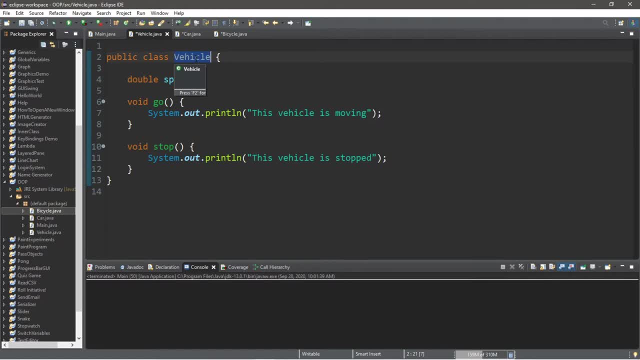 So this vehicle class is like an ancestor: It's giving an inheritance to its descendants, meaning its attributes and its methods. So let's create a car object and a bicycle object to see if this theory is true. So let's create a car Car. we'll name it. car equals new car. 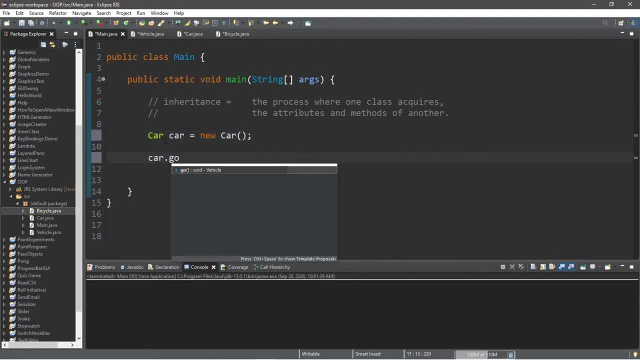 And we'll have our car use the go method And it says this vehicle is moving, but we didn't list anything within the car class. So how can this be? How is that possible? Well, since car is a descendant of the vehicle class, it receives everything that the vehicle class has, meaning a speed and a go method and a stop method. 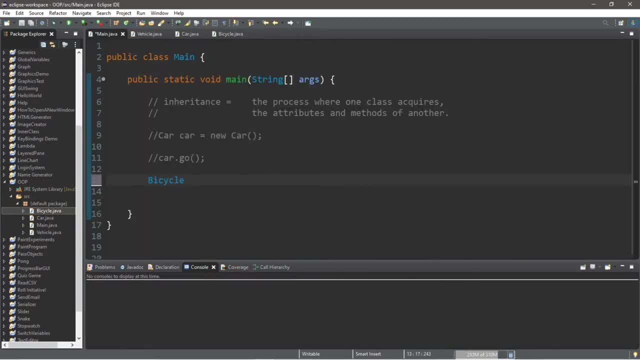 Now let's create a bicycle object. So bicycle, let's call this bike, equals new bicycle, And we'll have our bicycle object. use the stop method, Which it apparently has, even though we have nothing listed within the bicycle class, And then both the car class and the bike class should have their own speed variable. 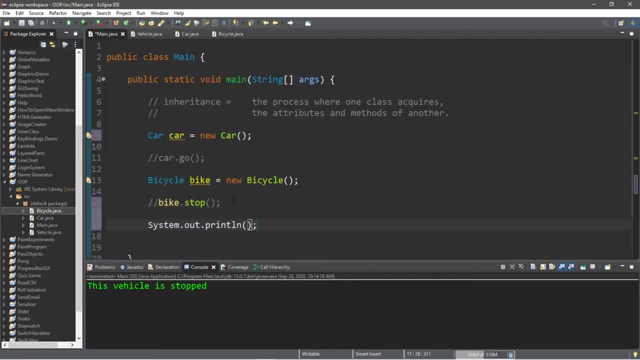 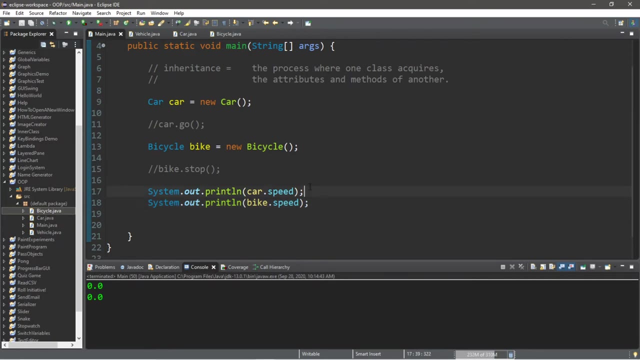 So let's also display that. So let's systemoutprintln carspeed, And the same thing goes with our bike object: Systemoutprintln bikespeed. And they should both be zero, Which they are. So that's one of the benefits of using inheritance. 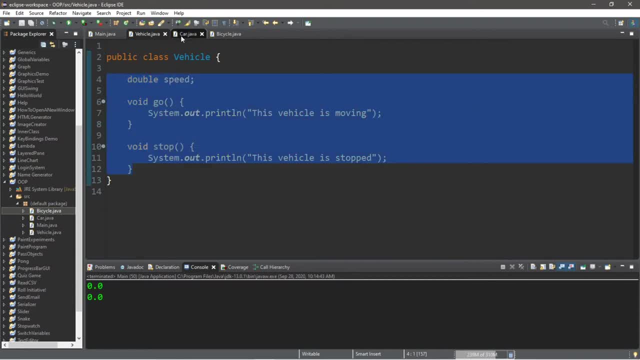 For one. we do not need to list all of these attributes and methods twice Now. another benefit of this is that we can have this car class and this bicycle class have their own unique additional attributes and methods, Since not all cars and bicycles are the same. 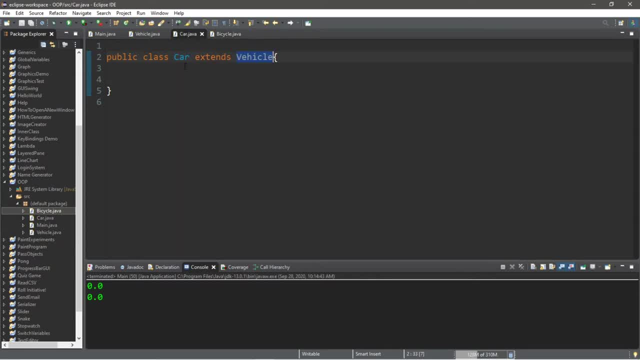 They are two completely different objects. So we can say that cars will also have a perhaps number of wheels, So int wheels, And we'll set this to four, And then bicycles will say int wheels equals two, And then with cars they have doors. 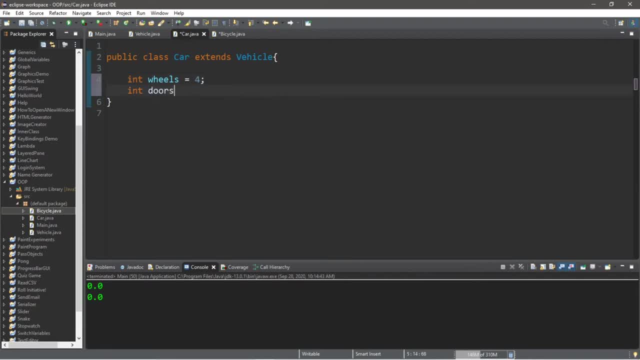 We can create another variable for that: Int doors, And this could be like two or four, I'll just say four for now. And then bicycles don't have doors, But they do have pedals, So int pedals, And this will be two. 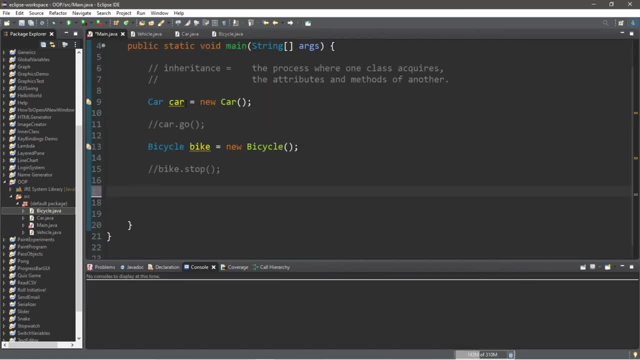 And if we head back to our main method, Let's display the amount of doors that cars have And the amount of pedals that bikes have. So we can do this with a print line statement- Car dot doors- And we'll display this. 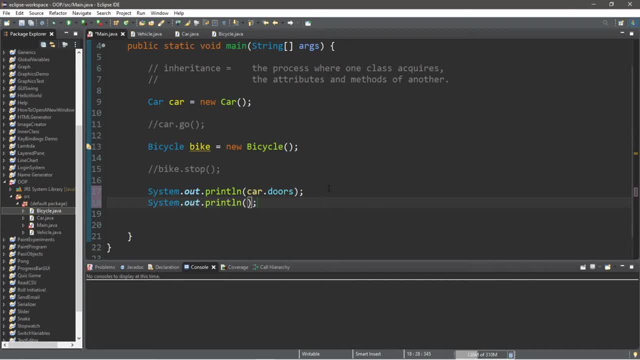 And we'll do the same thing with bikes, But display the number of pedals: Bike dot pedals. So our car has four doors And our bike has two pedals. Now, these attributes are unique to the car class and the bike class, So cars don't have pedals. 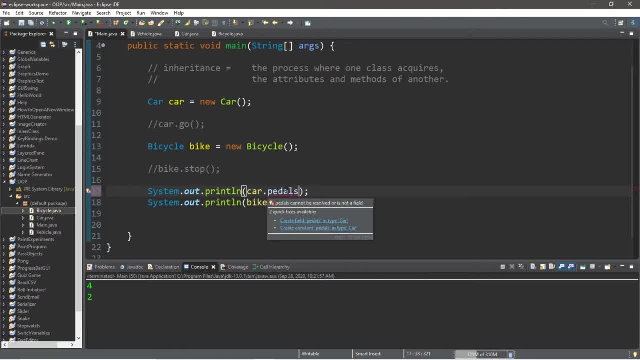 And if we try and access the pedals variable, Well, it's not going to be recognized. And our bike doesn't have doors, So this variable isn't recognized either. So when might you want to use inheritance? Well, for one, you'll probably want to use it if you have more than one class. 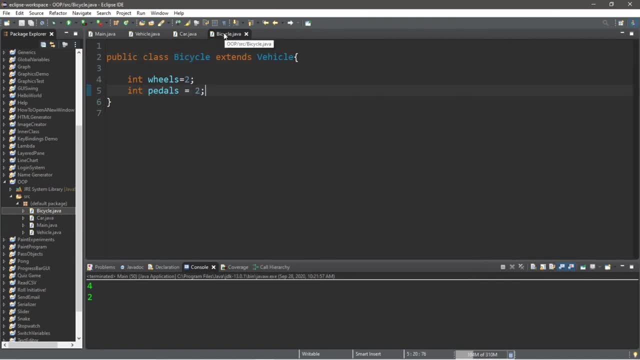 So if you have two separate classes, For example cars and bicycles, You can list everything that they have in common, Such as a speed, Some ability to move or go And an ability to stop, And then we can just list that within another class. 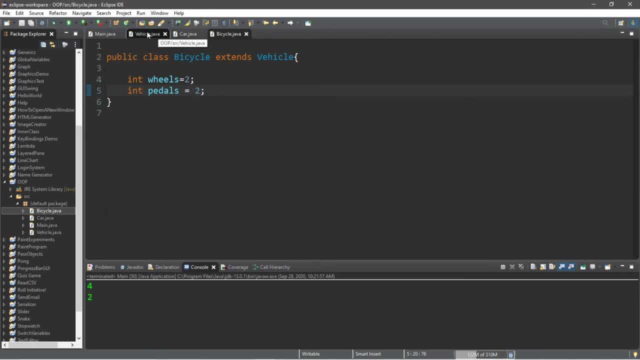 And have our car class and bicycle class Just receive everything That this vehicle class has, Because this is what they all have in common. So that's the basics of inheritance. If you would like a copy of all this code, I will post all of this in the comments down below. 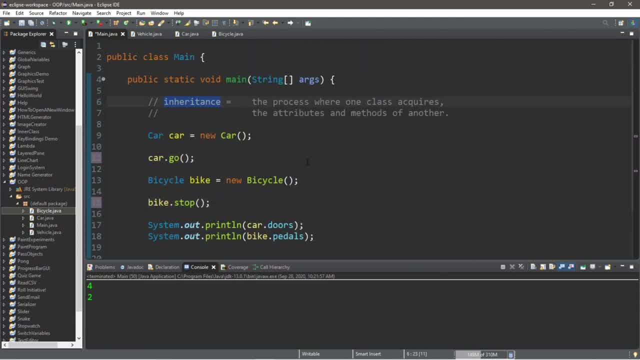 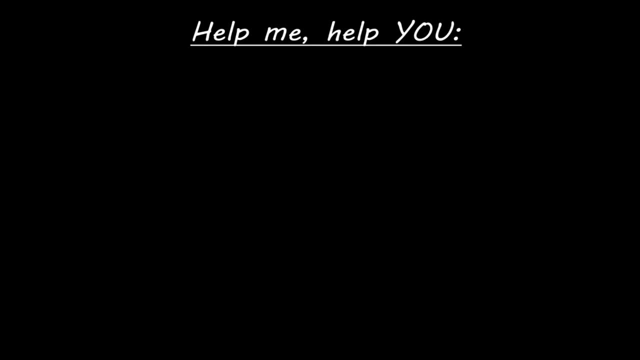 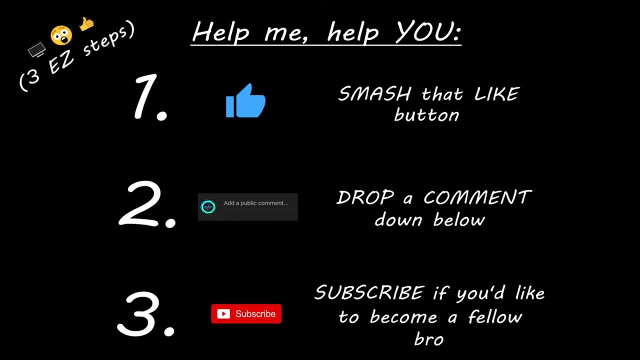 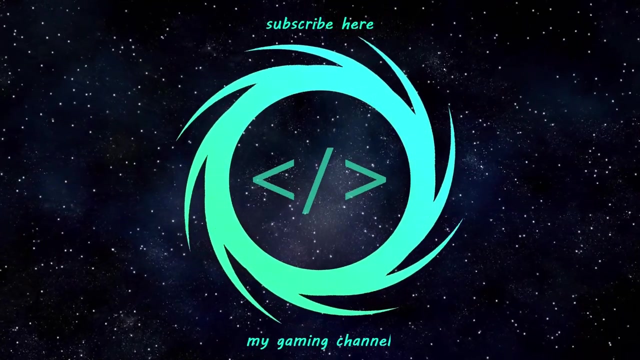 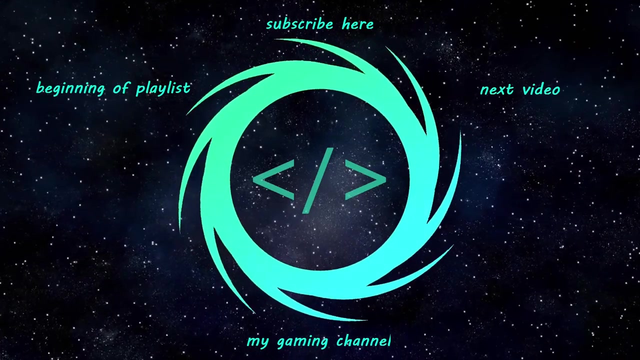